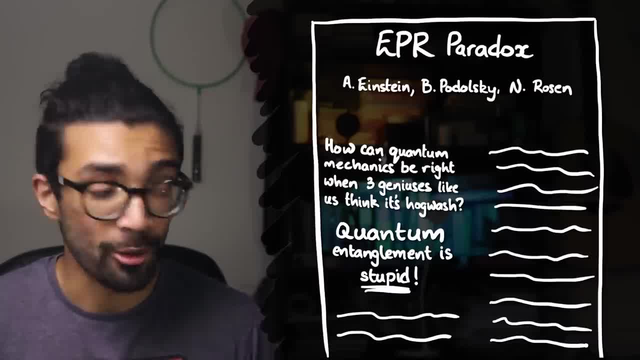 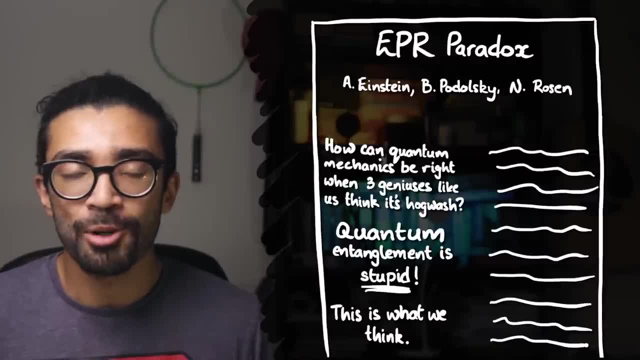 Anyway. so in this paper that Einstein, Podolsky and Rosen wrote, they basically showed the ludicrousness of quantum mechanics, The ludicrousness of quantum entanglement, or so they thought. They especially had a problem with the idea that, in an entangled state, if we were to make a measurement on one of the particles, 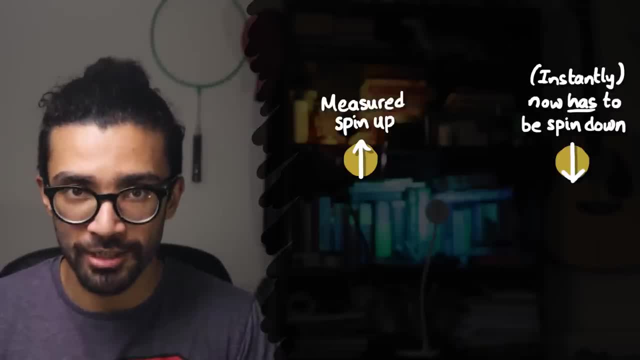 then we would have immediate, instant knowledge about the other particle, thereby causing a collapse of the wave function of this quantum system. To them, this seemed like instantaneous communication, The idea that we could know something about a particle that was very, very far away, instantly. 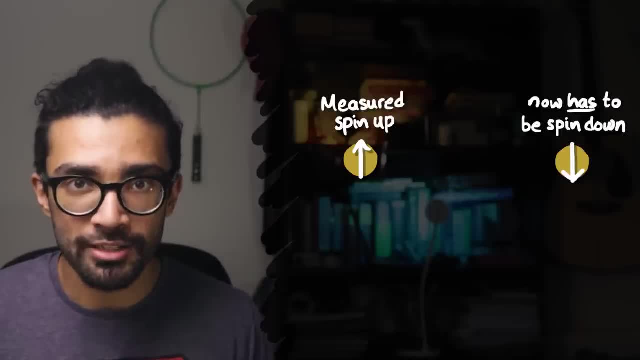 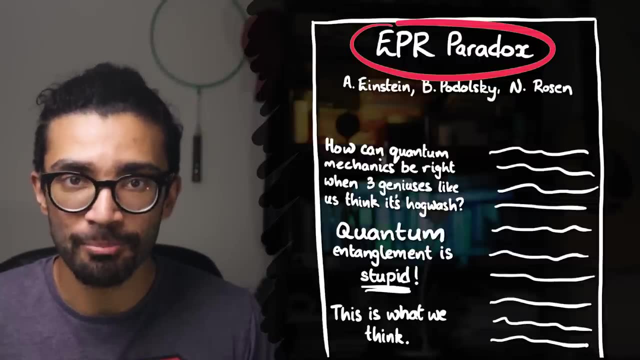 without even having to wait for light to come from that particle and reach us, simply because we'd made a measurement on it. This is what they said about quantum entanglement on the particle near us. This scientific paper that they wrote therefore brought up the EPR paradox. 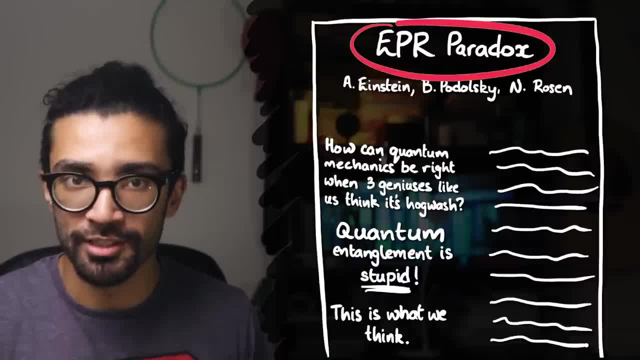 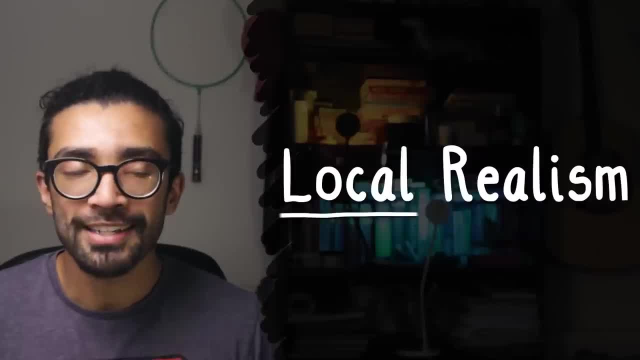 To understand the EPR paradox we first need to understand the assumptions that EPR made in their scientific paper about our universe. They assumed local realism. Locality is this idea that, say, two particles are separated by a large distance in space. They cannot instantaneously communicate with each other because it takes time for the information from one particle to reach the other, and this is restricted to travelling at the speed of light at most. And this assumption actually makes a lot of sense, given how successful Einstein was with his theories of relativity. 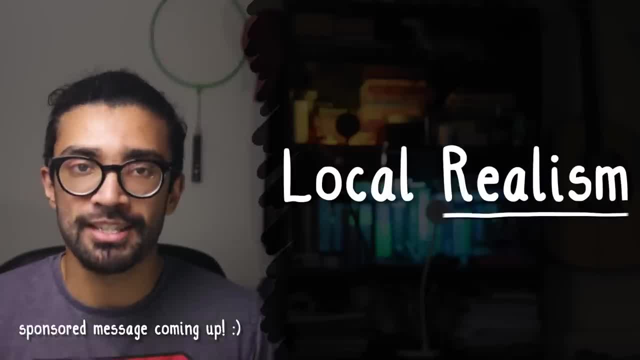 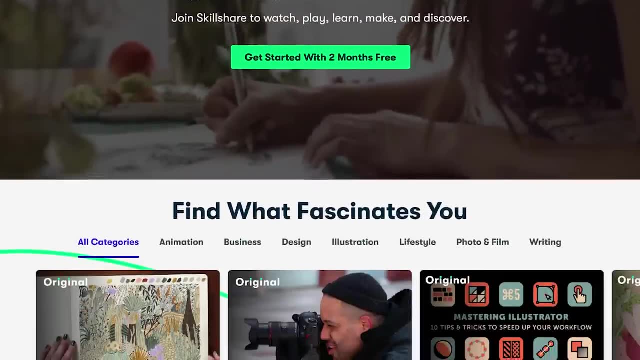 which made the same assumption. We'll come back to the meaning of realism in just a second, But before we do, I want to take a moment to thank this video's sponsor, Skillshare. Skillshare is an online learning community where you can find a large number of inspiring classes. 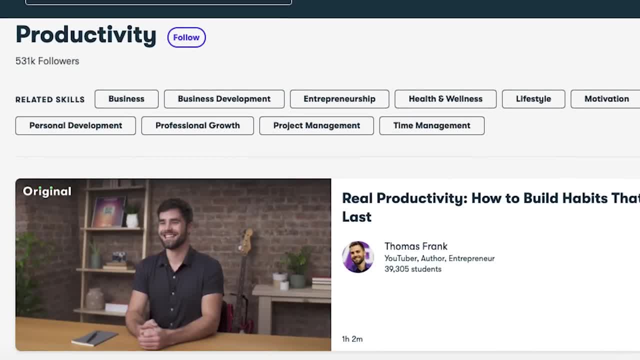 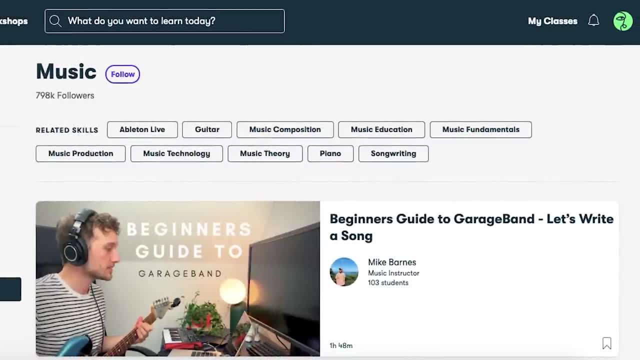 Focusing on topics such as productivity and lifestyle, to building a career or business, to learning creative skills in areas like music and so on. As many of you will know, I'm a huge advocate of having multiple passions in life and I've taken a few classes on Skillshare that have been genuinely eye-opening to me. 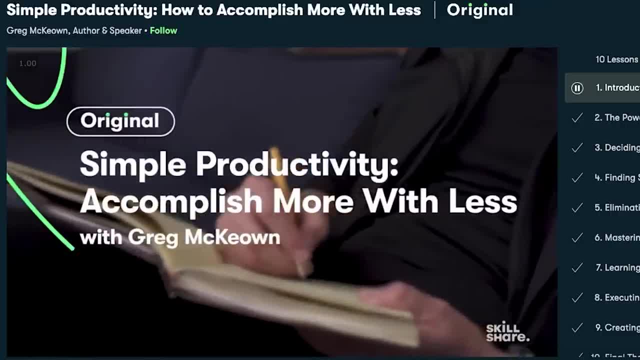 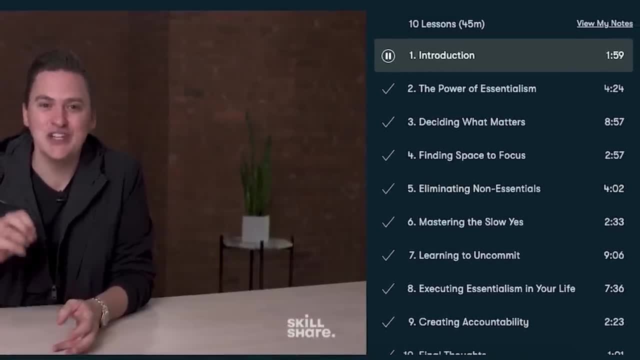 For example, I took a class called Simple Productivity- How to Accomplish More with Less- by Greg McKeown, and he provided some simple and easily actionable ways in which we can boost productivity. Skillshare has a large number of classes to choose from, and it's all about learning, so there are no adverts. 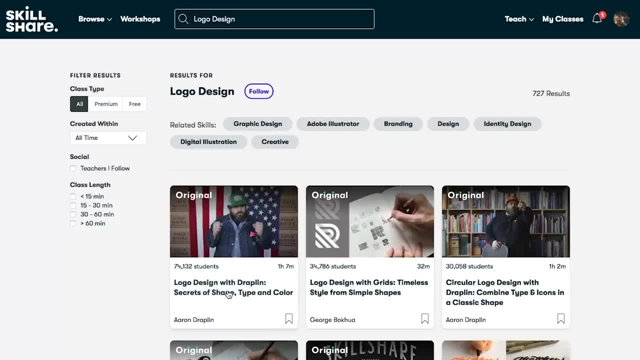 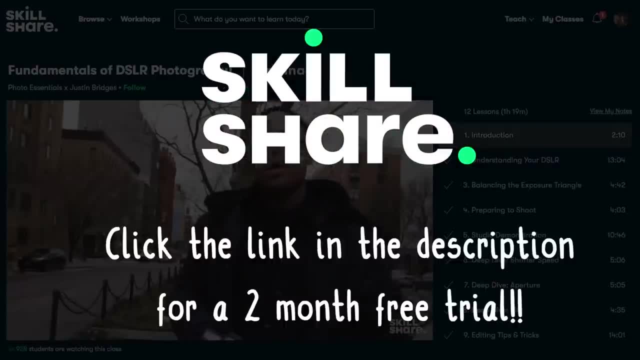 Most classes are less than an hour long, which means it's not a major commitment to sit down and learn something new, And Skillshare costs less than $10 a month when you get an annual subscription, However, the first 1,000 people to click the Skillshare link in the description below will get two months for free. 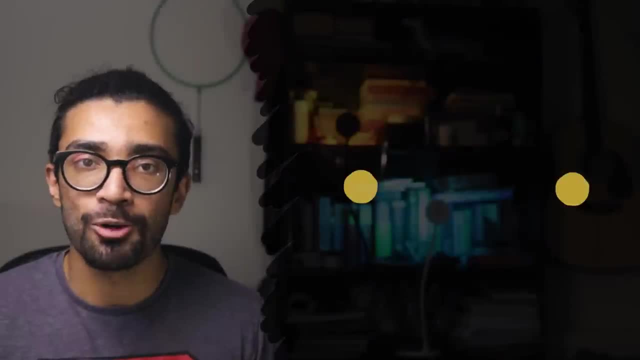 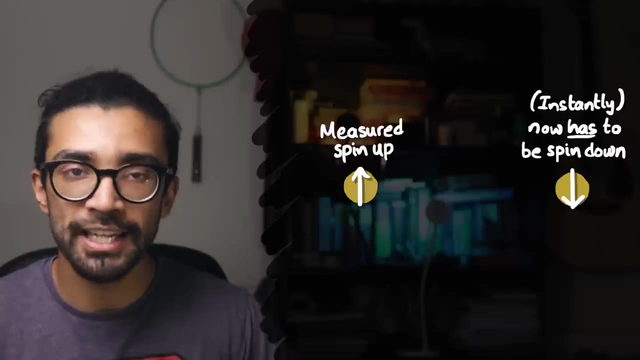 Big thanks again to Skillshare for sponsoring this video. Let's take a look at how quantum theory dealt with entangled particles. As we've already mentioned, quantum mechanics suggested that making a measurement on one of the entangled particles would immediately cause a change, a collapse, of the wave function, if you will. for the second particle also. 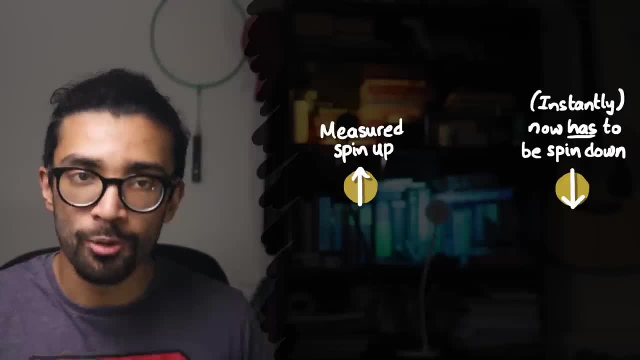 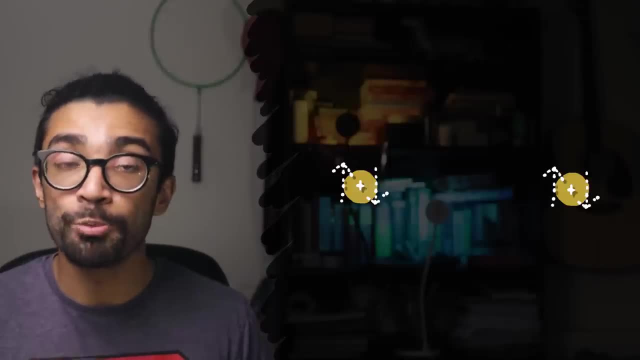 However, interestingly, quantum mechanics suggests that before we made any measurement on any of the particles, the system was in a sort of blend, a sort of superposition of all the different states it could be found in when we were to make a measurement on that system. 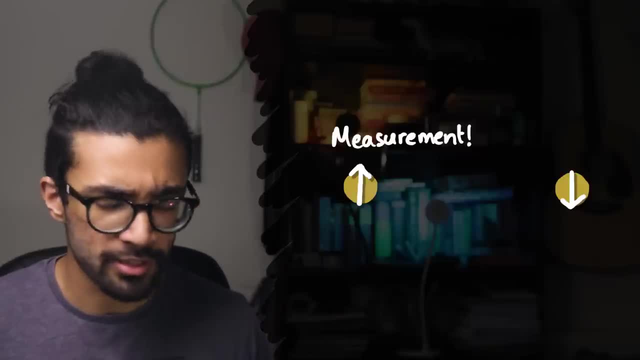 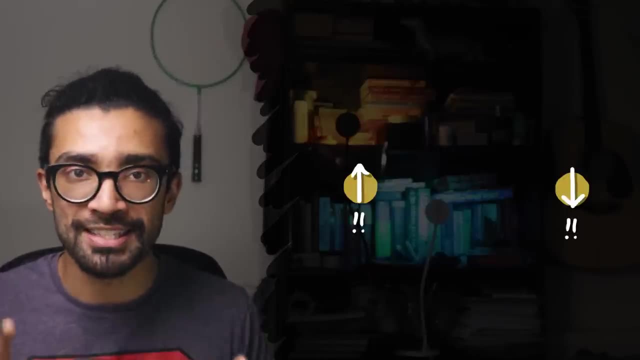 This is important because this is slightly different to our quantum system already being in a particular state and we just don't know what that state is until we make a measurement on that system. Those are two distinct ideas: This quantum mechanical idea that our system was in a blend of various different experimental results, essentially, 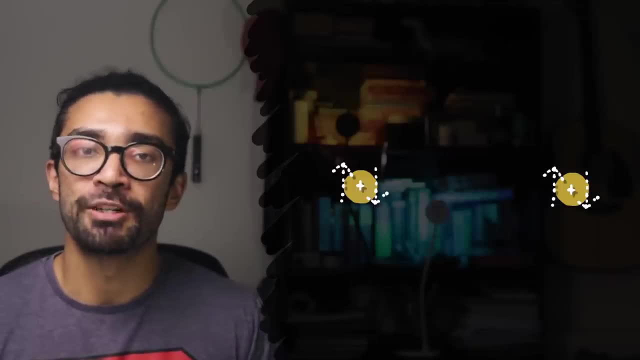 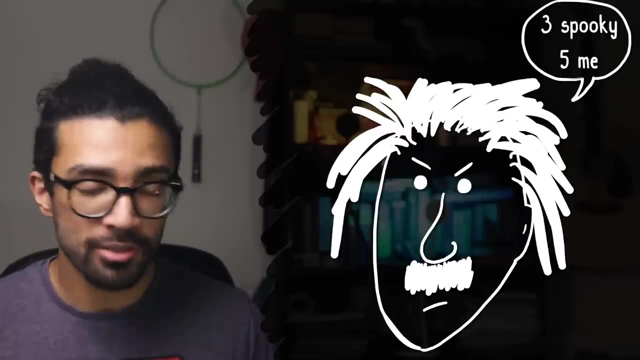 until we made a measurement on it. we discussed this idea multiple times in previous videos and, quite frankly, Einstein hated it. He called it spooky action at a distance, because supposedly a measurement on one particle could suddenly affect the other one as well. This is because entangled particles are described by the same wave function in quantum mechanics and they're essentially behaving like one big system. Now I suppose at this point you might be thinking: how can we tell the difference between a system that's in a blend of states before we make a measurement? 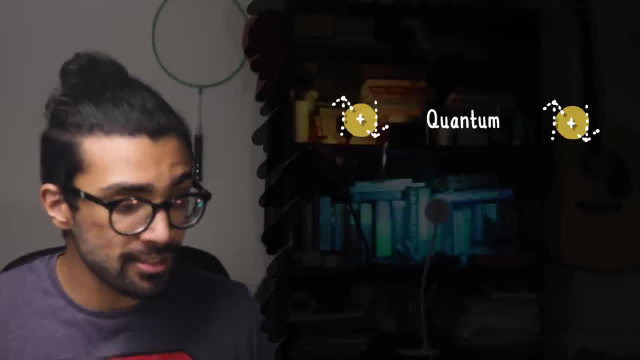 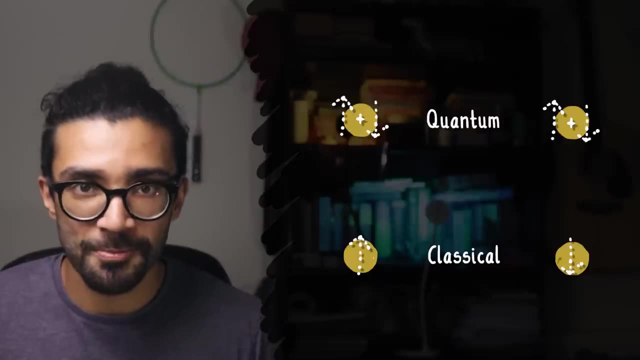 and then collapses into a state when we make that measurement, and a system that simply happens to be in a particular state that we don't know yet and we just find out what that state is when we make the measurement. Well, EPR actually suggested this second idea as a plausible explanation for what's going on with these weird states. 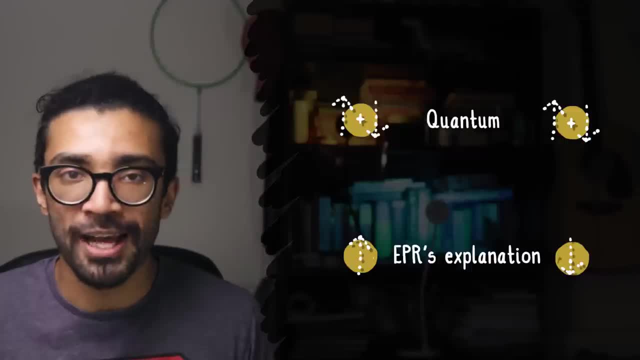 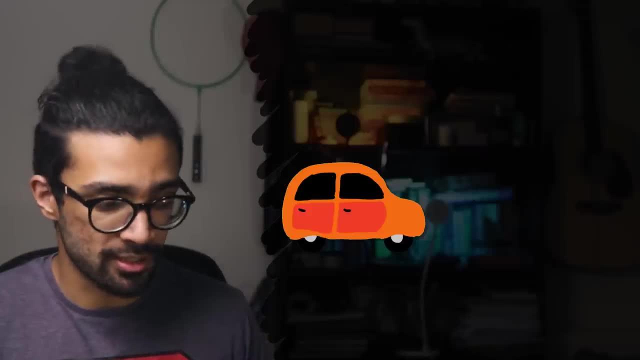 We'll understand this in more detail shortly, but first let's remember that we haven't talked about realism yet. Realism, sometimes interchangeably called determinism, is this idea that if we've got a system and we have all possible information that we can have about this system, 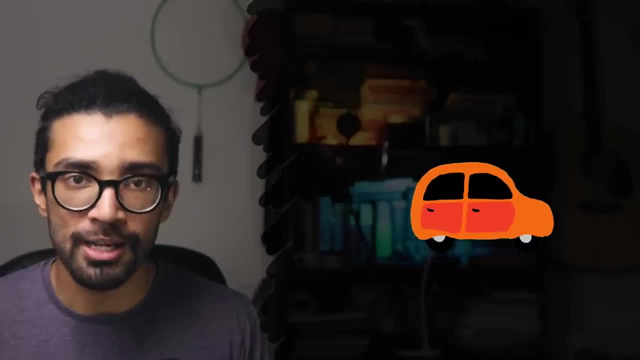 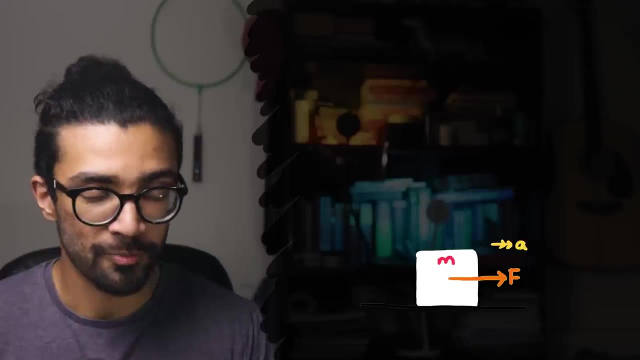 then we'll be able to work out exactly how it behaves as time progresses. All of physics was deterministic up until quantum mechanics came in and ruined the party. Newton's laws of motion assumed, for example, that if we knew the mass of an object, 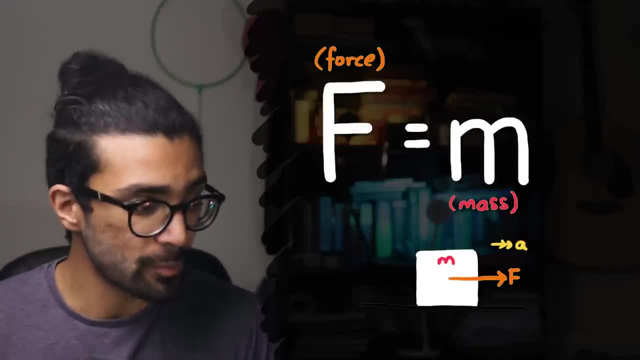 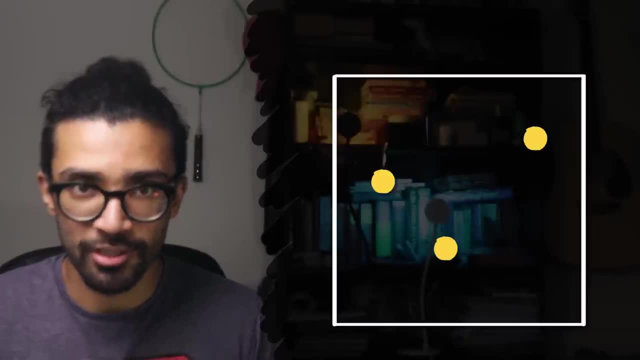 and we knew the force that was being exerted on that object, then we could precisely and accurately calculate the acceleration of that object. Or, for example, if we had a box containing a lot of gas molecules, Let's say we knew their exact positions, velocities and masses at one point in time. 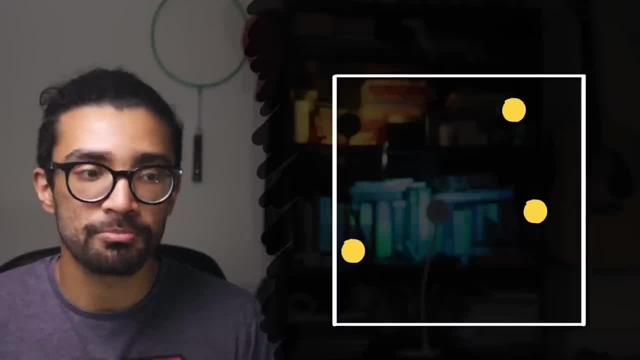 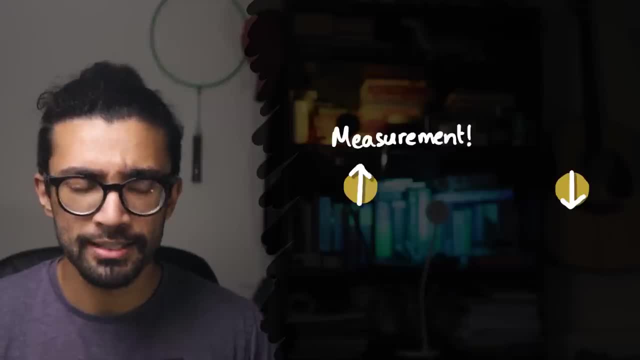 then we should be able to calculate exactly how the gas looks at some later point in time. It's also worth noting here that this seeming lack of realism or determinism in quantum mechanics is what brings in this whole argument about consciousness being important to our universe. 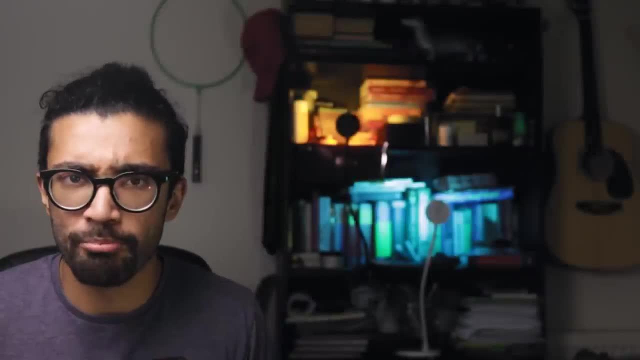 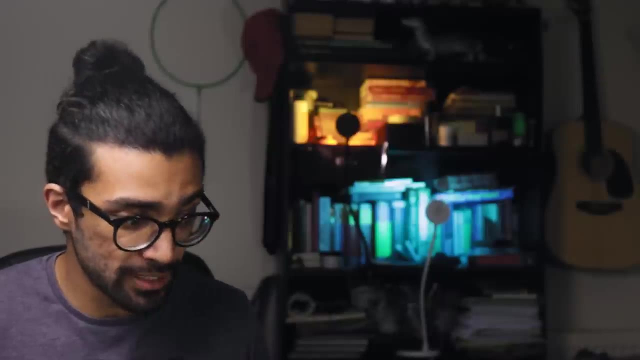 and without consciousness, nothing exists, because who's there to measure things and who's there to observe the universe? Some scientists believed that this is exactly what was happening. Other scientists believed that it was the actual interaction between the measurement device and the system that we happen to be measuring. 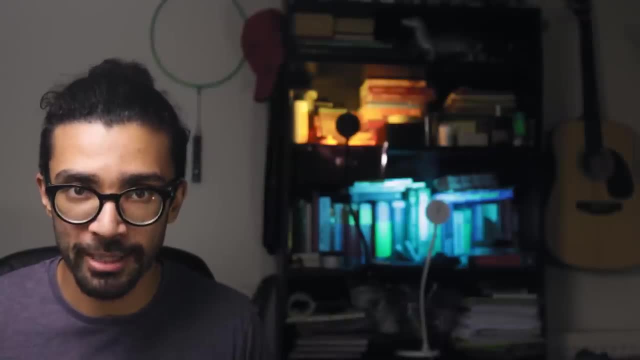 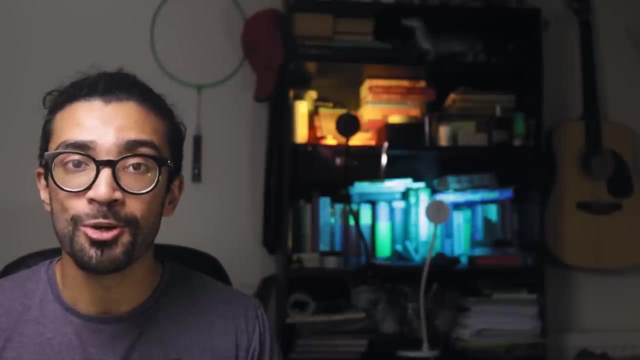 that was causing the collapse of the wave function, and this is still a hotly debated topic. But it has also meant that people have taken this consciousness idea into the realm of pseudoscience. My advice to you is to always be wary of someone who definitively tells you. 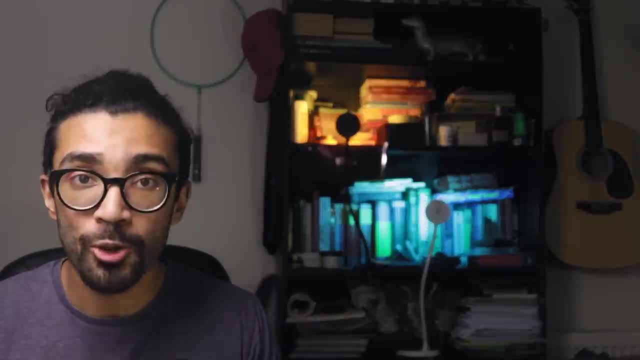 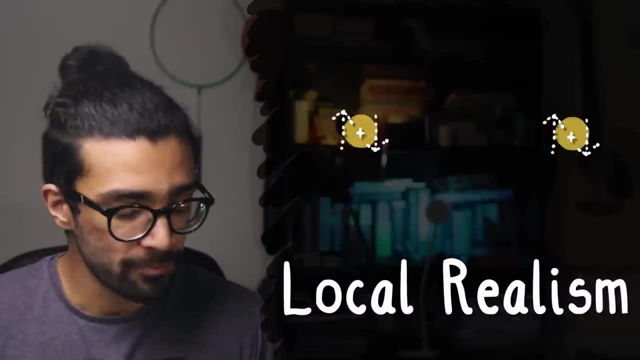 that consciousness is the key to the universe. We don't know that that's true yet. so if somebody suggests that that is 100% the case, Yeah. Anyway, coming back to EPR's problem with quantum mechanics, Now if we imagine that these two particles in the quantum entangled state, 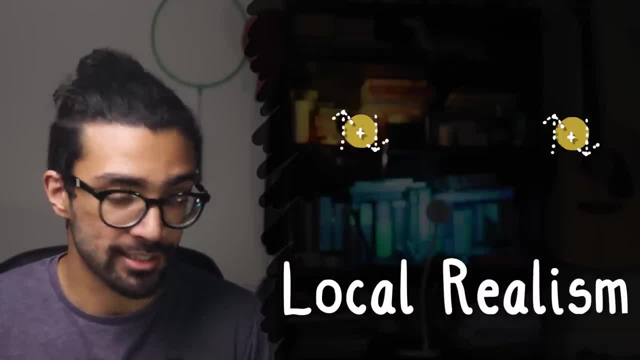 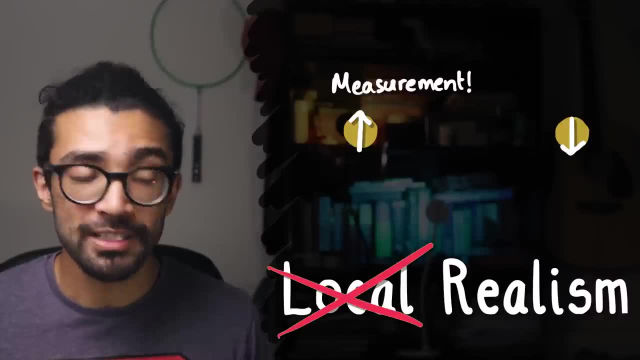 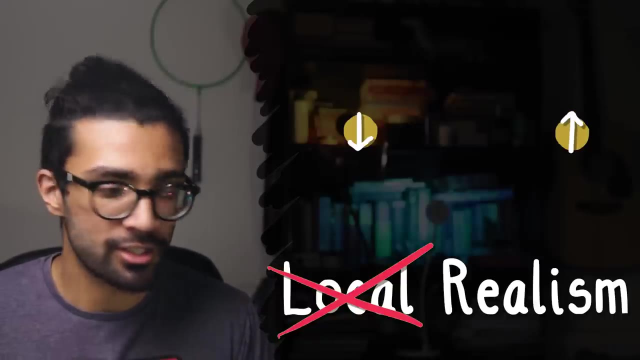 are separated far enough from each other that it takes light a considerable amount of time to get from one to the other, then this instantaneous collapse supposedly breaks locality. Also, this idea that the system collapsed into a particular state when we made a measurement and it had some amount of randomness as to which state it collapsed into. 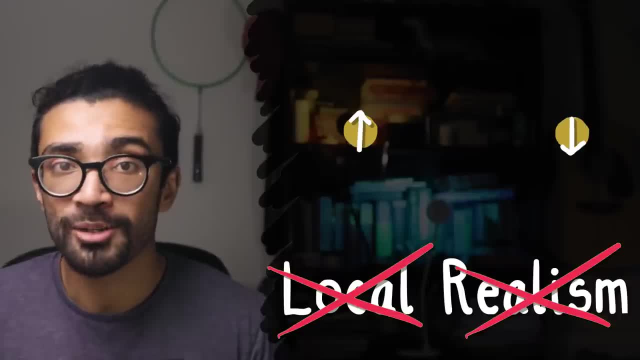 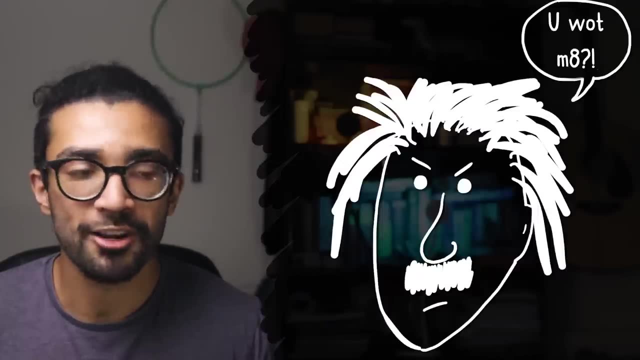 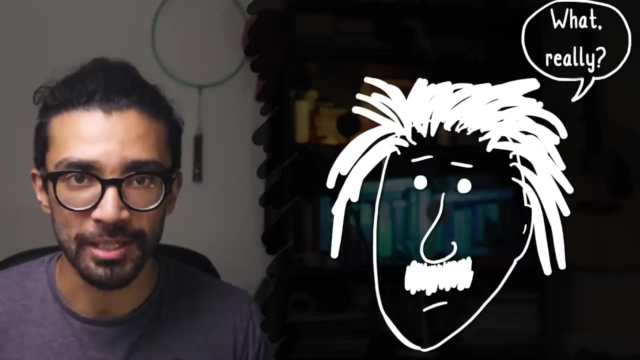 really didn't work with realism or determinism. Their whole argument was that the universe seemed to be local and deterministic, and quantum mechanics broke these. So WTF? This is how they justified to other scientists that quantum mechanics must be wrong. We now know that they were wrong at least partially, if not completely. 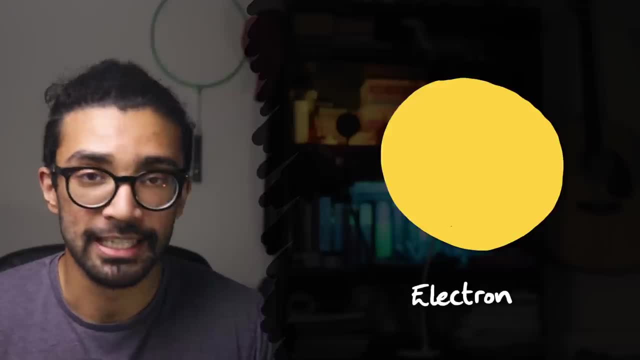 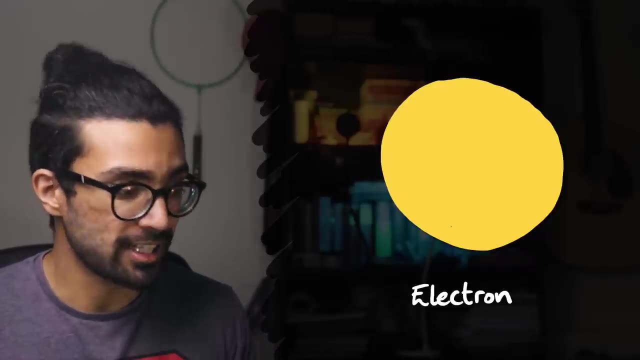 Let's once again imagine that we're measuring the spin of, say, an electron. We've already said that the two measurement results we could find are spin up and spin down. But what I haven't mentioned yet is that we measure the spin of a particle in a particular direction. 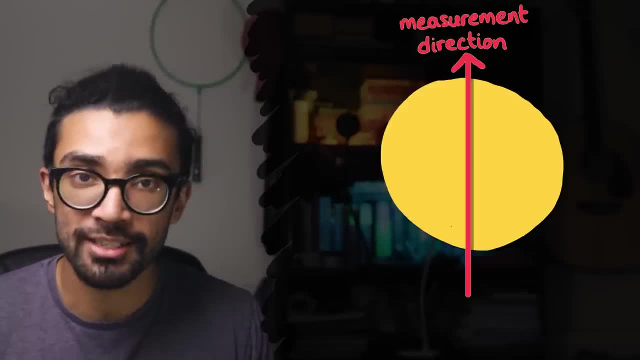 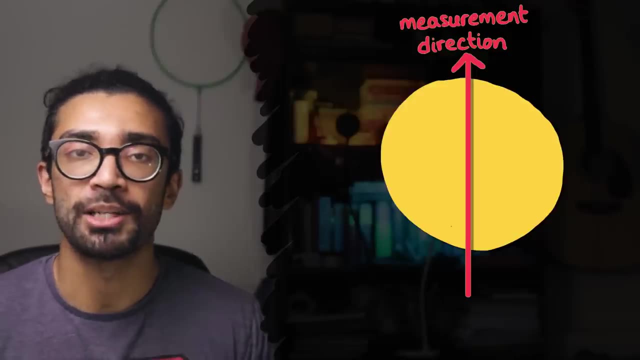 There's a reason spins are given arrows to describe them, because they are vectors. Essentially, what we're choosing to do is to measure the spin of an electron, say, in the upward direction, And we will always find the spin of an electron to either be pointing in that same direction. 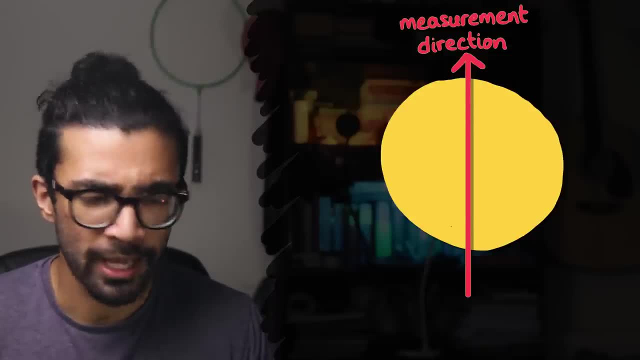 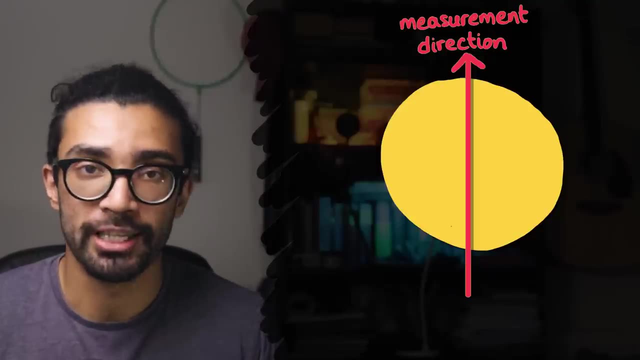 or pointing exactly against it. That's just how spin behaves. We're not going to go into too many details about spin. Check out this video if you haven't seen it already. But the important thing is that we have some way of measuring something about our system. 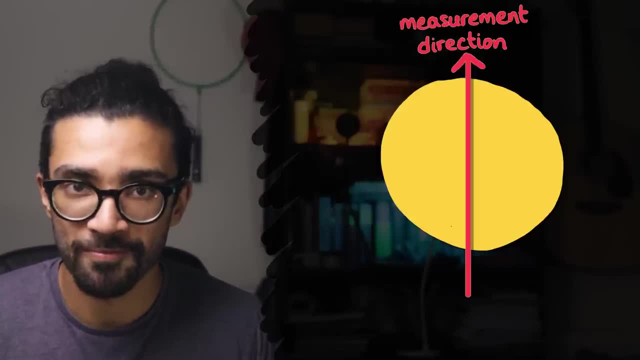 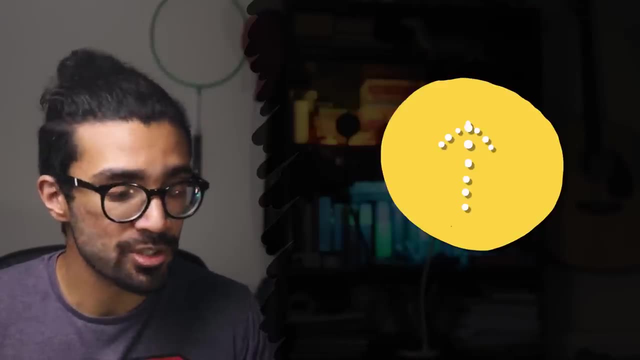 And we make a measurement in a particular direction. Now, why can't we say that the system, this electron, is already in, say, the spin up state, before we make a measurement, and then, as soon as we make a measurement, we just find out that it's in the spin up state? 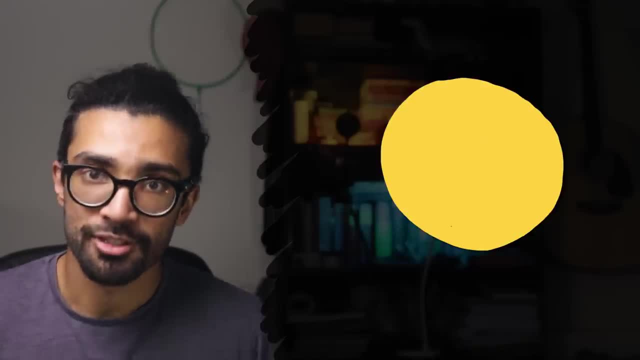 Well, EPR believed this to be true. The issue that they had to resolve came up when we had to measure the spin of this electron in different directions. Now, let's say that the particle's spin, before we made a measurement, was just in the spin up direction. 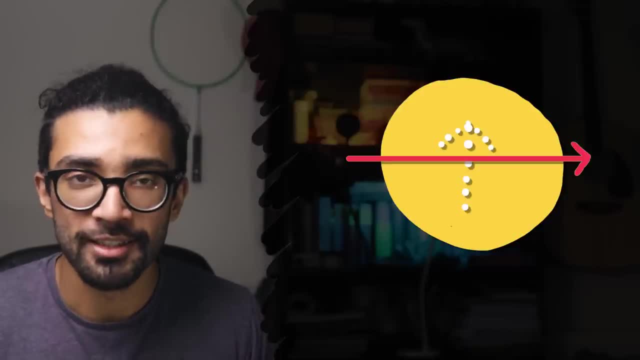 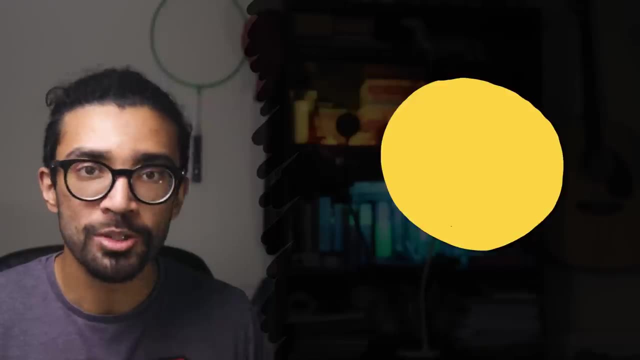 And we chose to make a measurement in, say, this direction. What would we find as our experimental result? Would we measure aligned or anti-aligned? And this is where we see two conflicting hypotheses about how the system may behave. One was quantum mechanics and the other one was the one laid out by EPR. 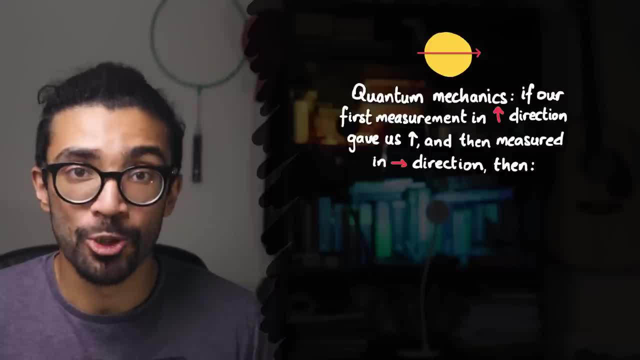 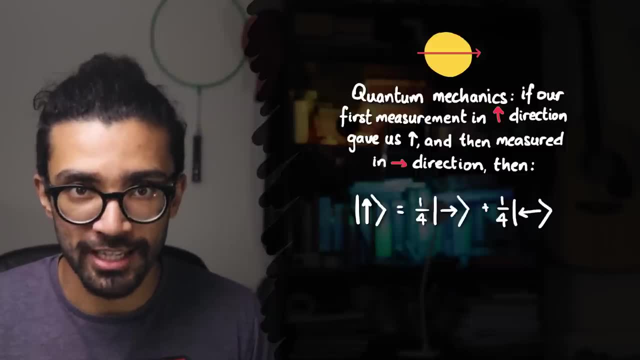 Quantum mechanics suggested that measuring in a different direction would not be a problem, because we could easily just write a spin up state as some linear combination of a spin right and a spin left state, And then we could work out the probability of finding spin right and the probability of finding spin left. 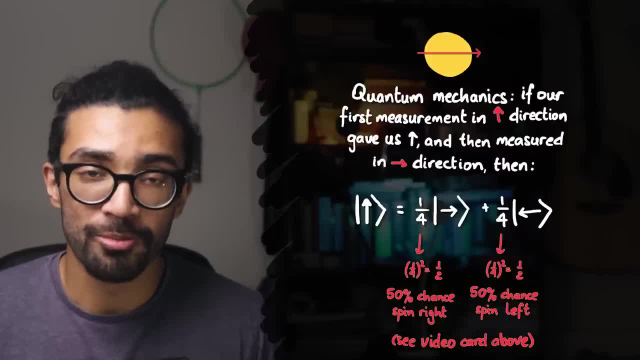 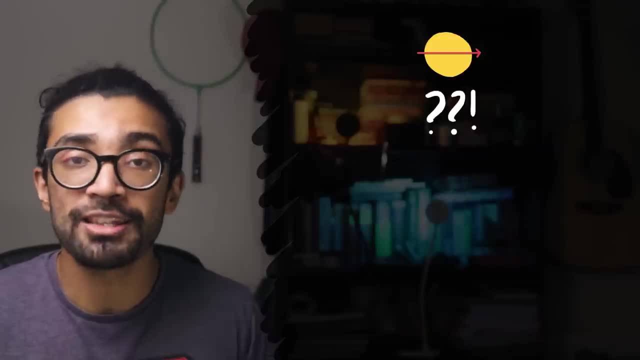 and it would just fall into one of these two states with their given probabilities. EPR suggested something different. EPR suggested that there was something built into the system, something that we couldn't access, maybe due to our lack of understanding, maybe because that's just how the universe was. 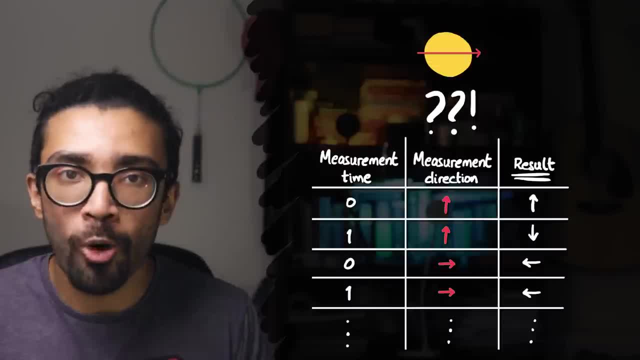 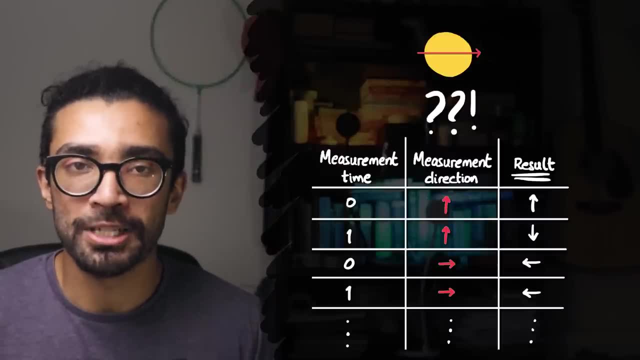 and this thing that was built into our system would tell the system what result to display when we made a measurement on it. This weird, inaccessible thing later went on to be called a hidden variable, And this was important for EPR because this did not break their assumption of determinism. 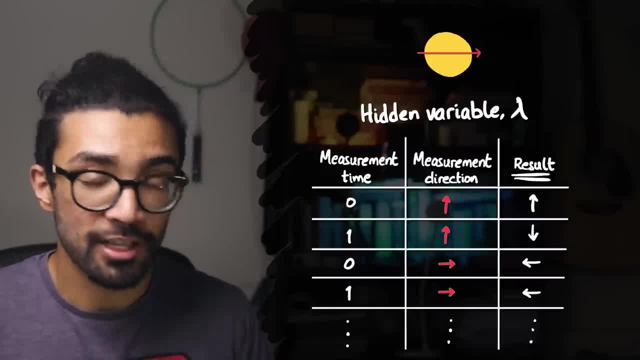 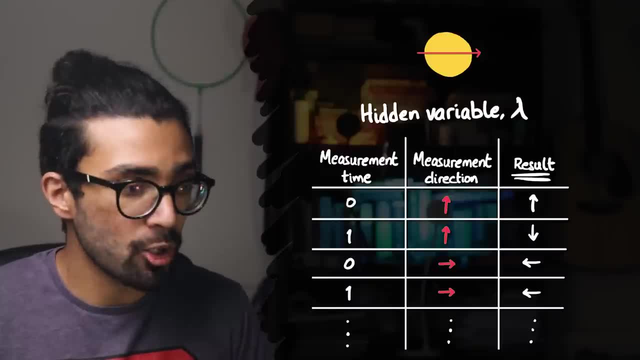 If there was something hidden away in the system that we couldn't access that resulted in the system giving particular results for particular measurement axes for particular times, then it's perfectly deterministic. There's no random collapse of the wave function going on. Locality is a little bit more of a difficult topic to discuss here.